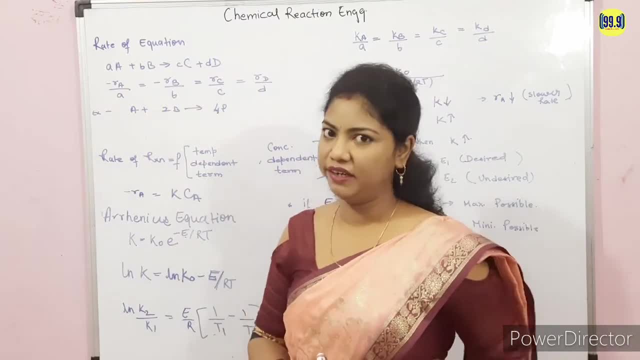 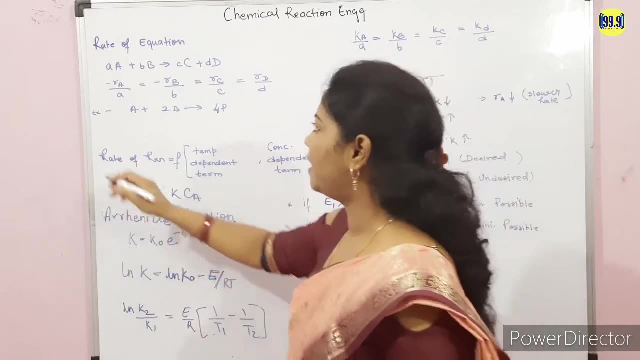 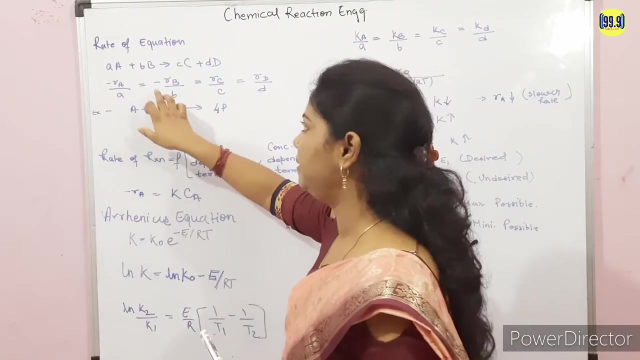 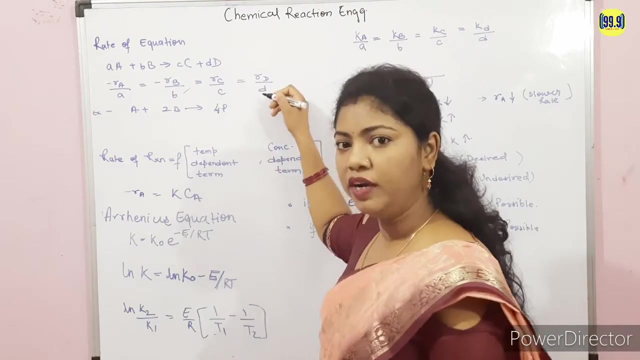 Here the small abc is the temp, is the statuometry coefficient. If we write the relation between the statuometry coefficient and the rate of reaction, it will be a minus. RA upon A is for the reactant, A for the reactant B will be minus. RB is equal upon B and for the product, RC upon C and the RD upon B. 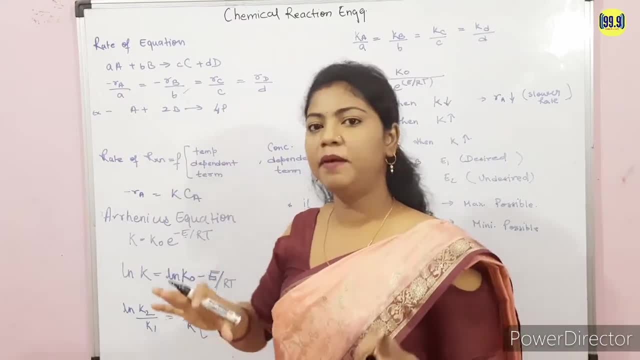 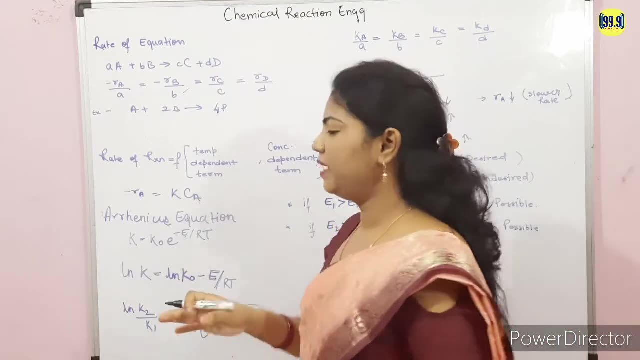 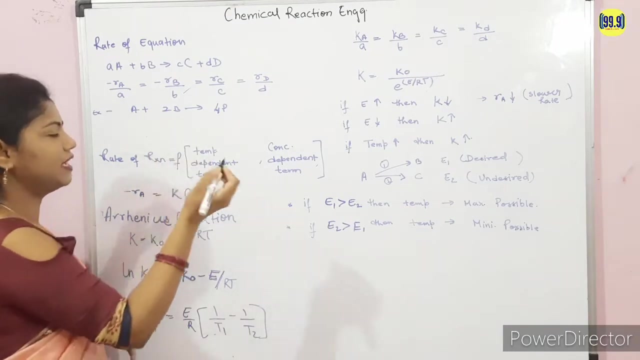 These are. we are taking negative sign for the reactant part of the component and we take positive rate of reaction for the product side. okay, So similarly, we are going to solve some one of the little bit. very simple equation, for example, is A plus 2B. 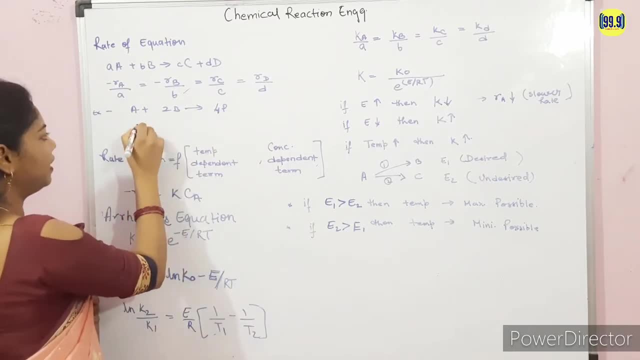 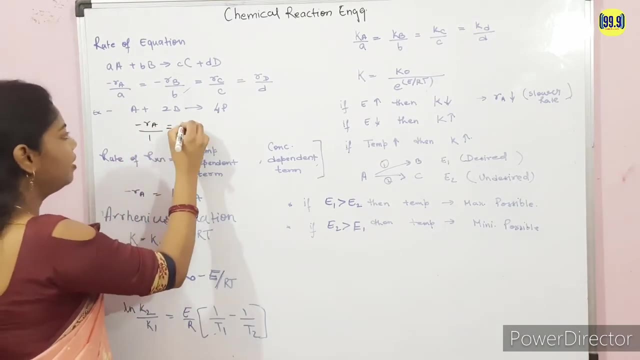 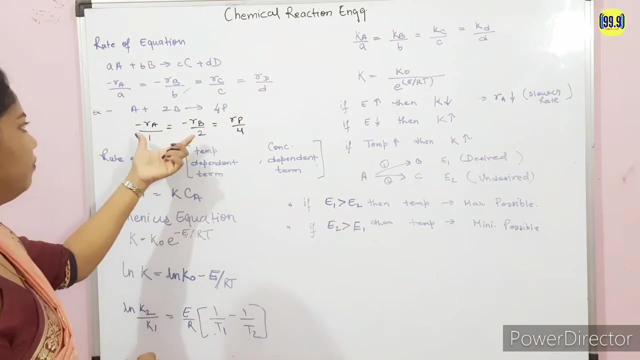 A plus 2B gives 4B. okay, In that case the rate of reaction relation between the statuometry coefficient and rate of reaction will be like that: minus RA upon 1, minus RB upon 2, is equal to RP upon 4.. So we are going, we are taking the negative sign for the reactant and the positive 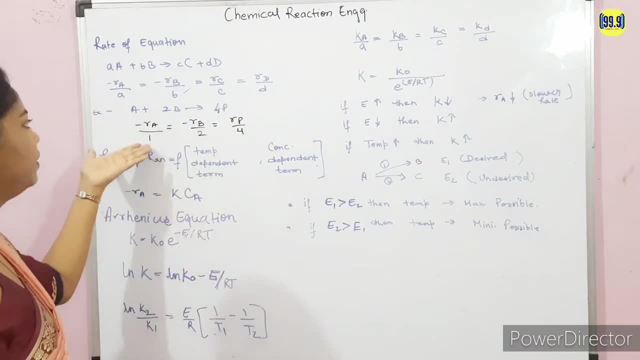 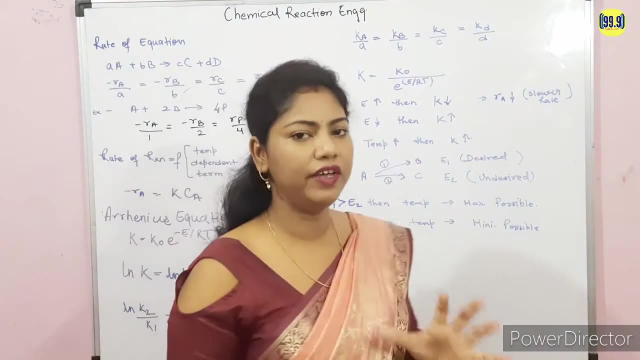 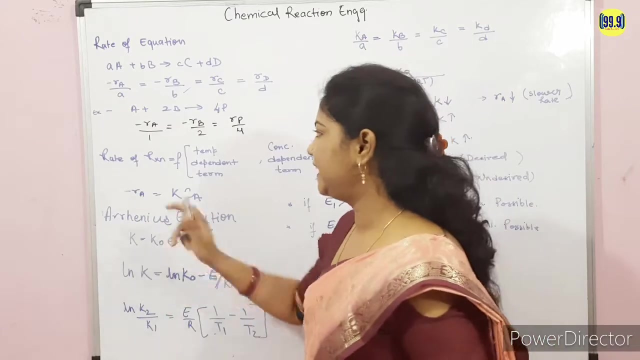 sign for product and we simply divide the coefficient- statuometry coefficient- with the rate of reaction. This is this is how we write the rate of reaction in terms of the relation between the statuometry coefficient. okay, So I already said that the rate of reaction is the function of the temperature. 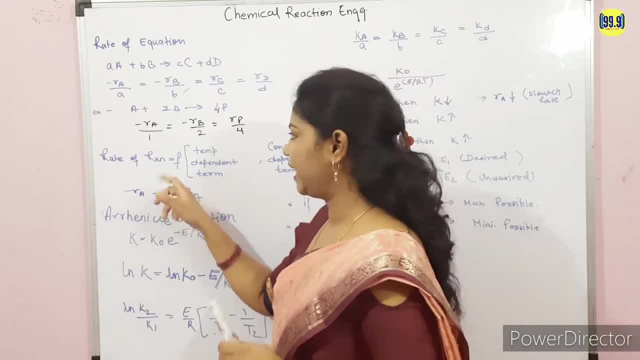 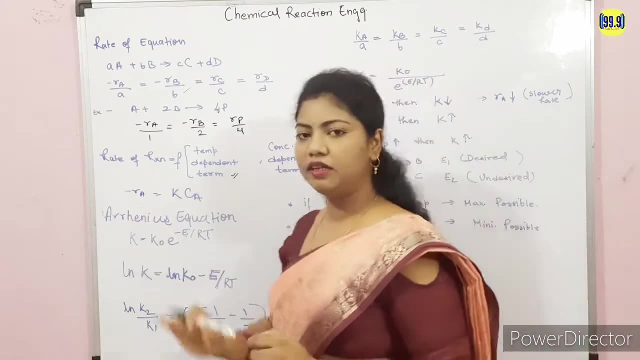 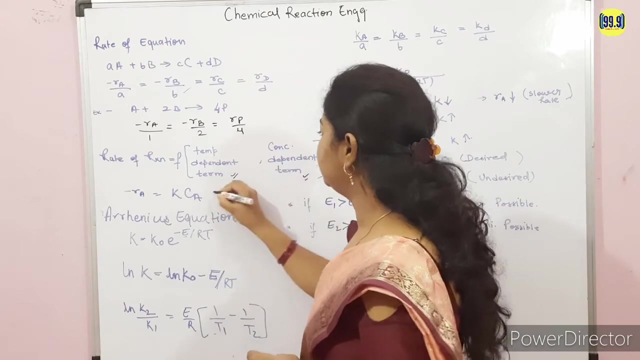 and the concentration. okay, So the rate of reaction is the function of temperature dependent term and the concentration dependent term. So we write it as a, as a mathematically like minus, RA is equal to KCA. okay, So this is the concentration dependent term and K is the temperature dependent term. and 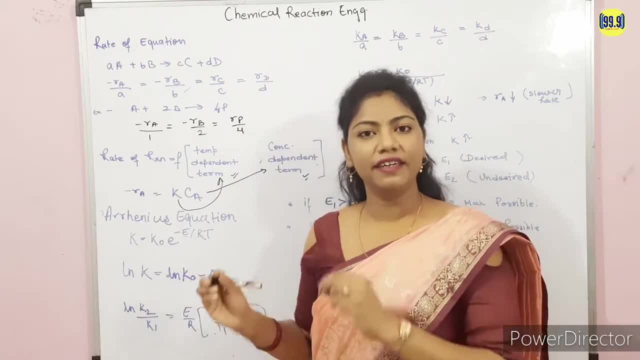 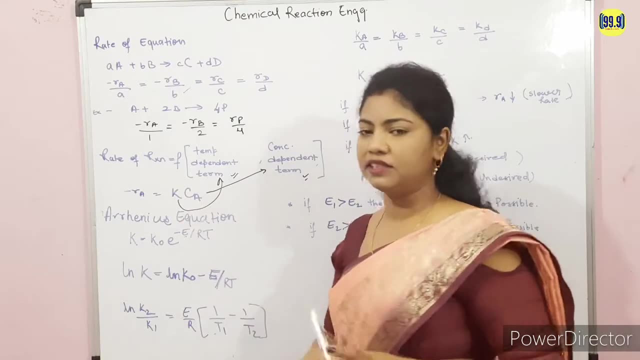 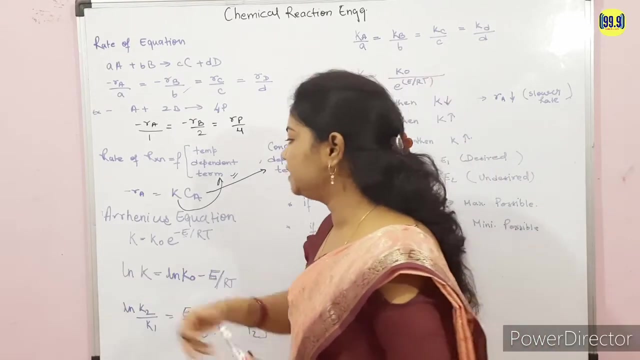 we call it as a reaction rate constant. okay, We call it as a reaction rate constant or reaction rate coefficient. So reaction rate constant is: is we get from the Arnie's equation, which is given by the K is equal to K, naught e to power, minus e upon RT. okay, This is very. 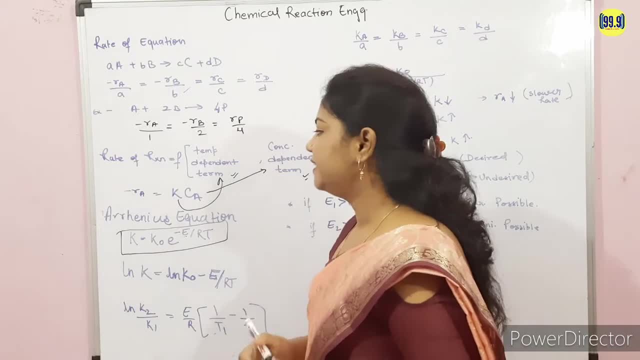 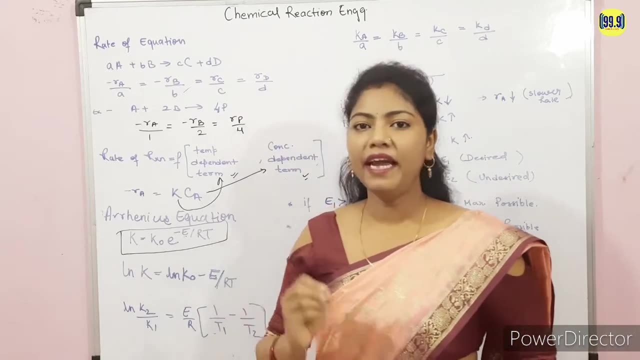 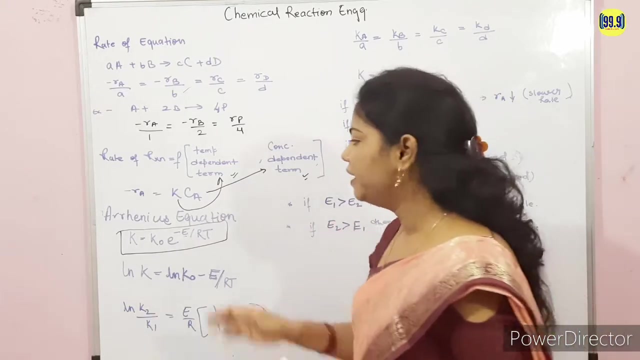 important equation, The enables the reaction of the Arnie's equation, that is, K is equal to K naught, e to power minus e upon RT. Here the K naught is the pre exponential factor, e is the activation energy and t is the temperature in Kelvin. okay, So what is activation energy? basically the activation. 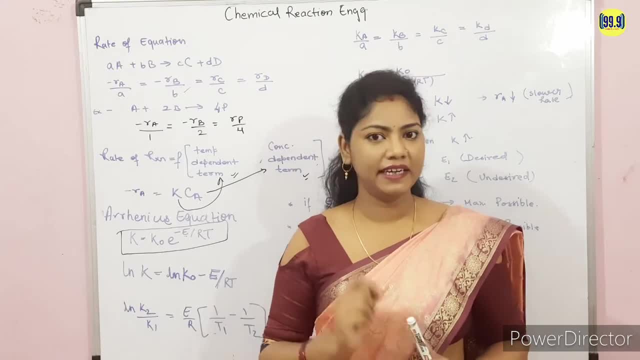 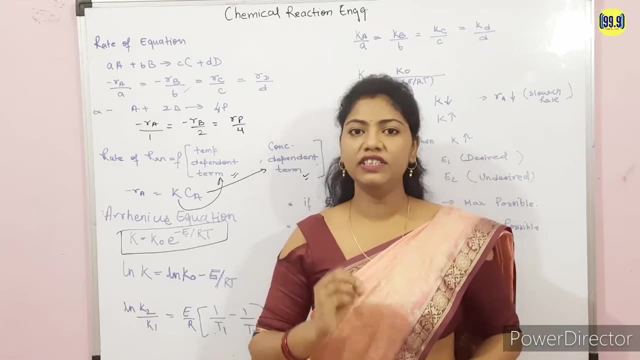 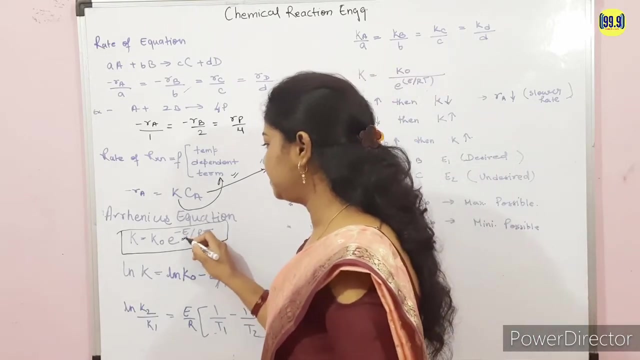 energy is the minimum amount of energy required by the reaction or reactant to start the reaction. okay, Questions. Question of energy which is required by the reactant to start the reaction? ok, So basically, we this term activation energy in this topic is very important and we are going to study the 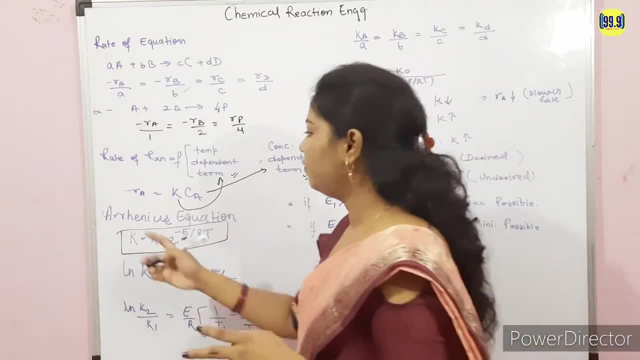 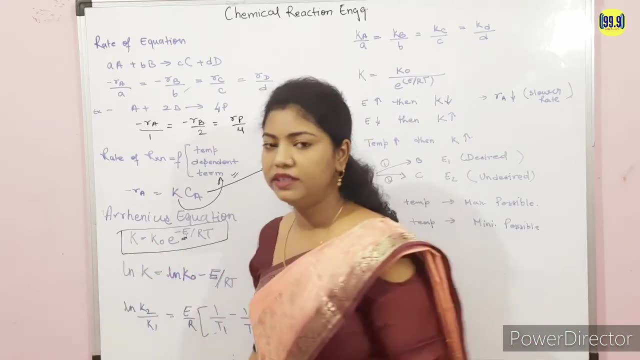 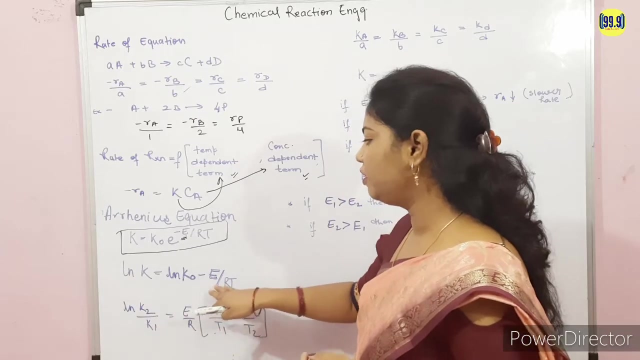 variation of activation energy with the rate constant, reaction rate constant. ok, So if we take logarithmic in the both, the both the side of the Arnie H equation, the equation become: ln k is equal to ln k naught minus e upon RT. ok, So this equation when, after the taking 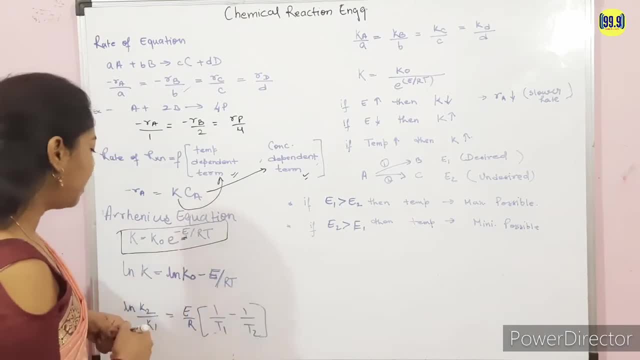 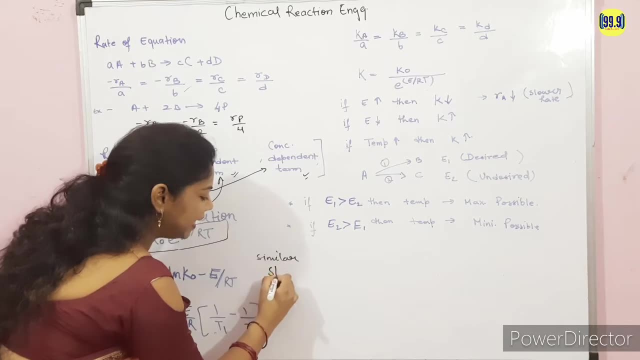 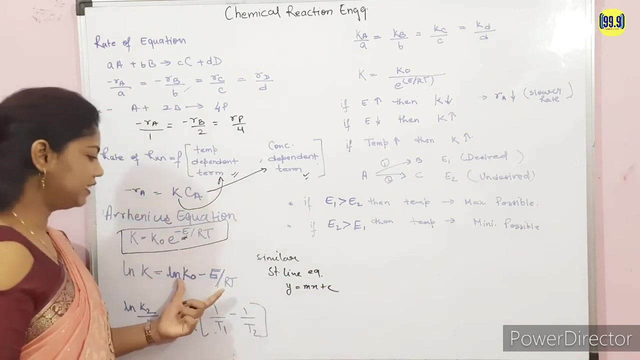 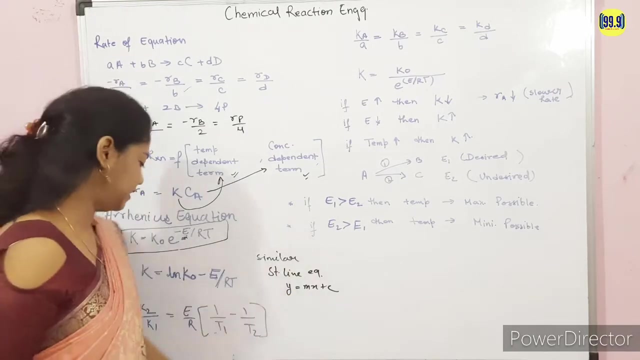 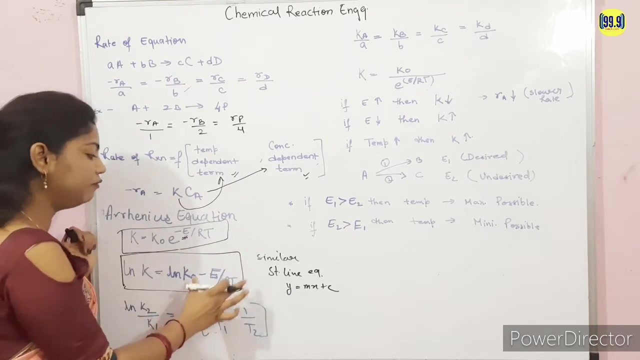 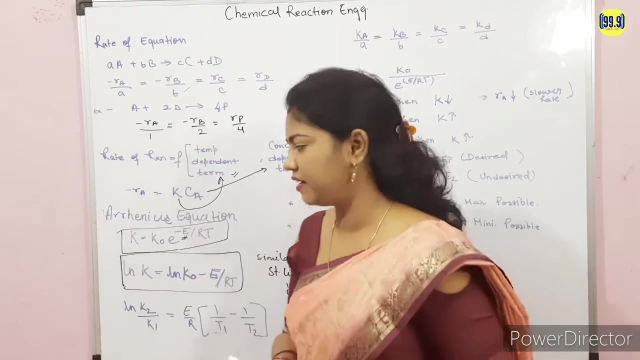 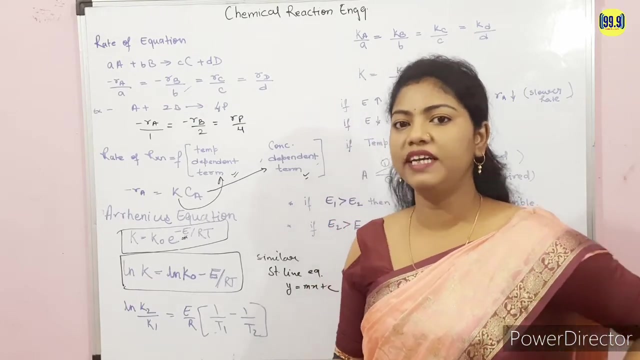 logarithmic, simple mathematical calculation, and we we get this equation which is similar to, which is similar to the straight line equation, that is, y is equal to mx plus c. You can see that this equation is very much similar to the Most similar to the: y is equal to mx plus c. So this is about this equation. Now, this is about the only this equation. when the we are considering only one temperature or concentration, same concentration. but if, if we have a different temperature condition, two different temperature condition, what will be the equation for that? but the concentration will be same in that condition, we apply the equation. 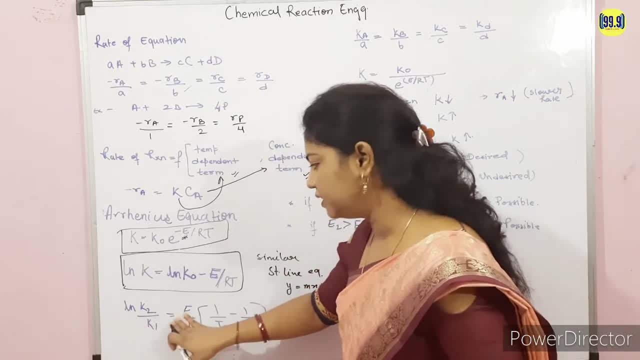 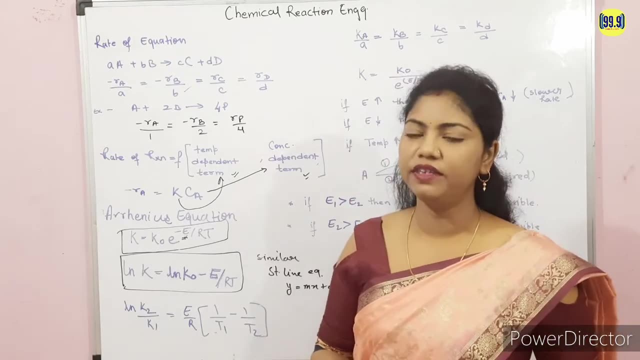 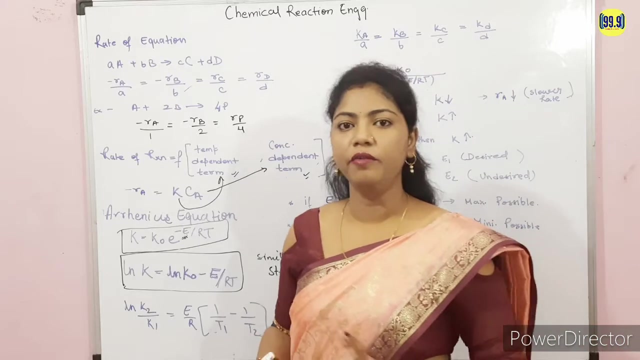 equation is like that ln K2 upon K1 is equal to E upon R, 1 upon T1 minus 1 upon T2.. Here the temperature we are going to take is two different temperature, but the concentration and same and the activation energy is same in the both the temperature condition. ok. So this equation is: 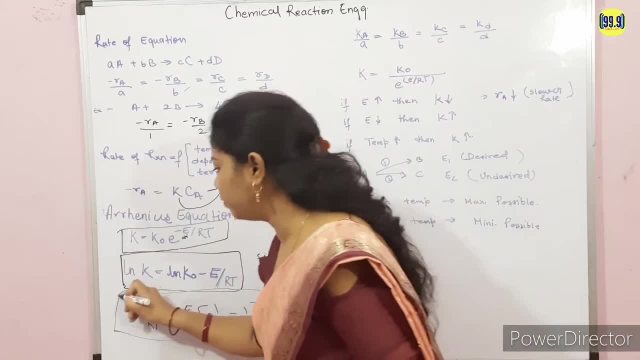 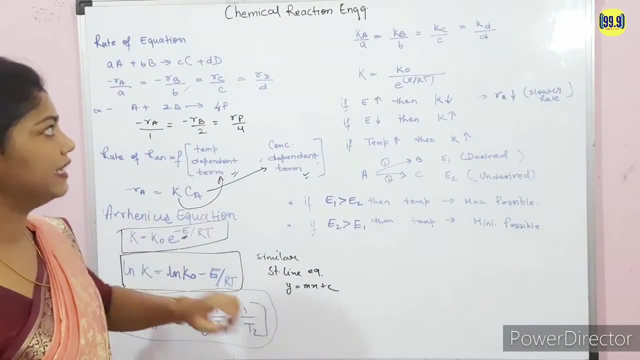 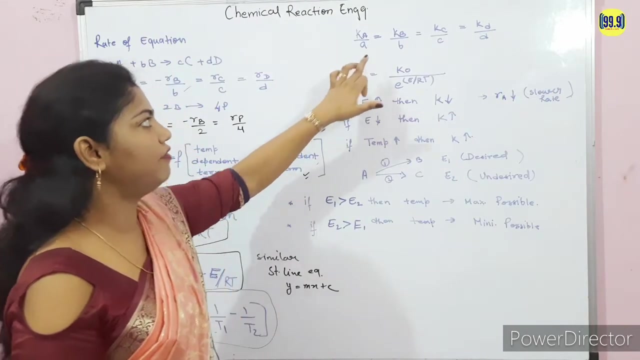 also very important in point of view of solving the gate: numerical, ok. So now the another thing we are going to study about the relation between the reaction rate constant and the stoichiometric coefficient. You can see here I have write it: Ka upon Ka is equal to Kb upon B. 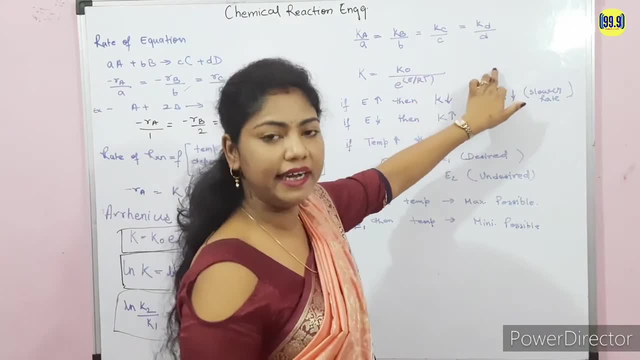 is equal to Kc upon C is equal to Kd upon D. This equation is almost similar to the equation of Kd upon D. So this equation is almost similar to the equation of Kd upon D. So this equation is almost similar to the equation of Kd upon D. So this equation is: 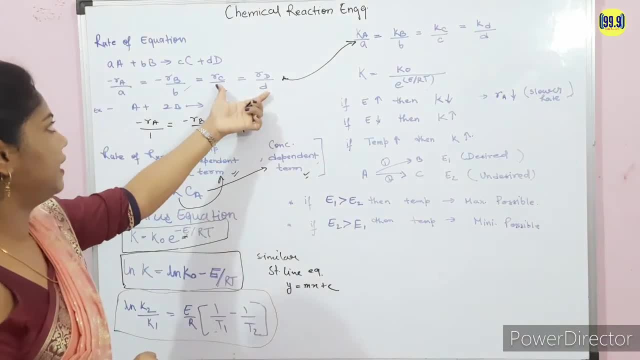 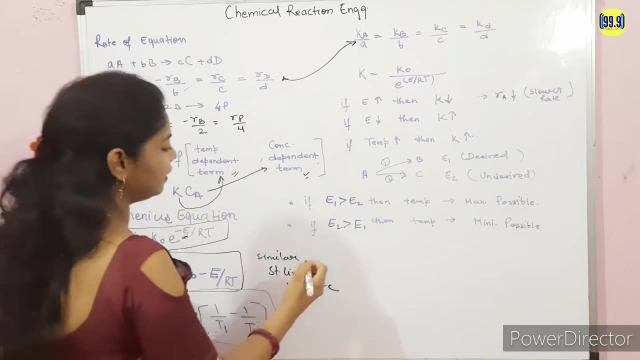 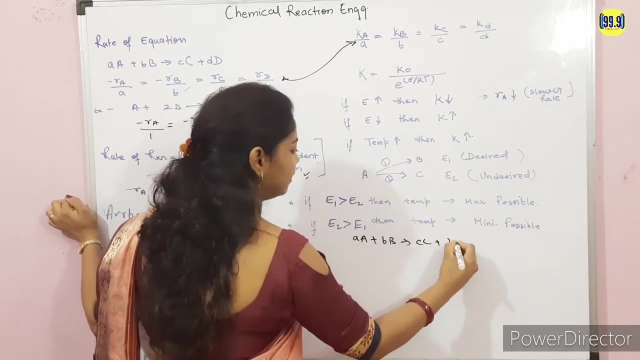 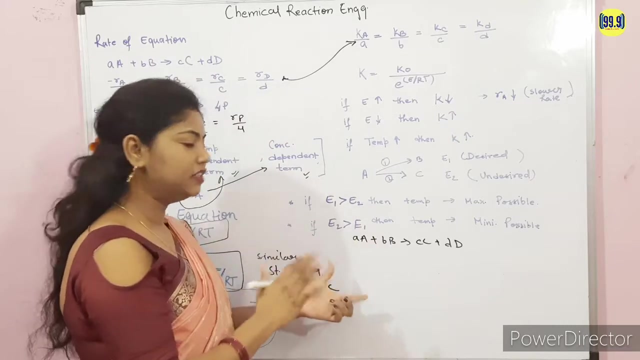 similar to the. this equation of the rate of reaction and how we get this reaction, this type of equation like: suppose we write: we have a reaction Aa plus Bb plus Cc plus Dd. ok, We have a reaction like that. So we can write the rate of reaction of the each of the component, like Ra is. 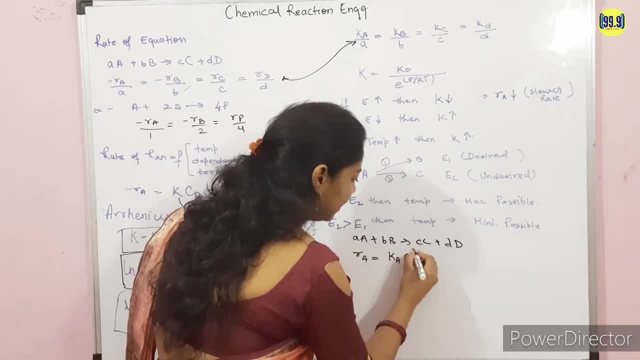 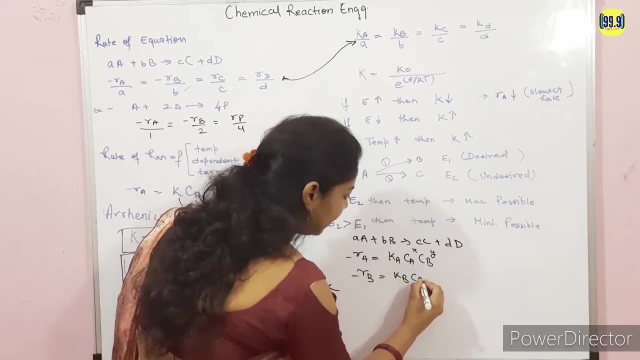 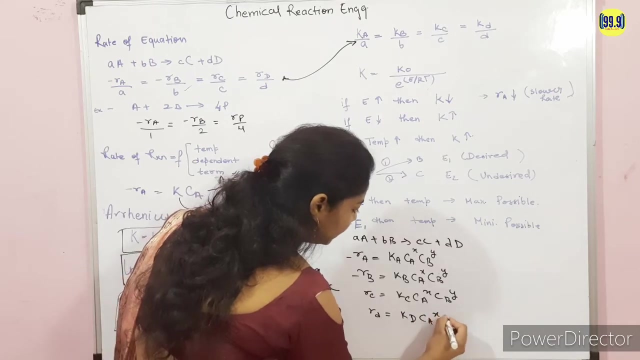 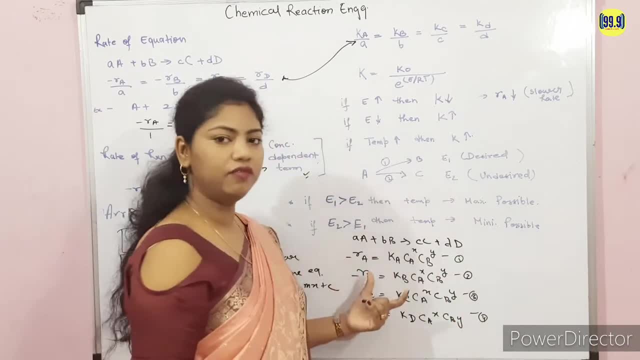 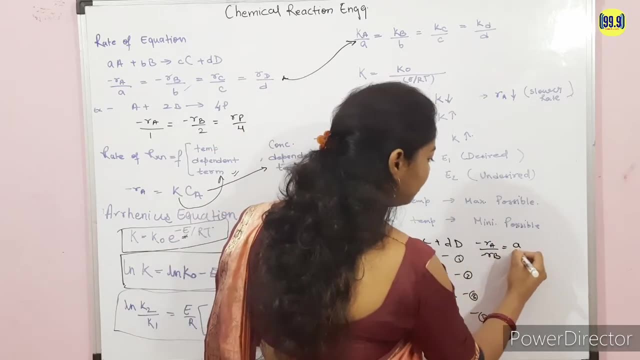 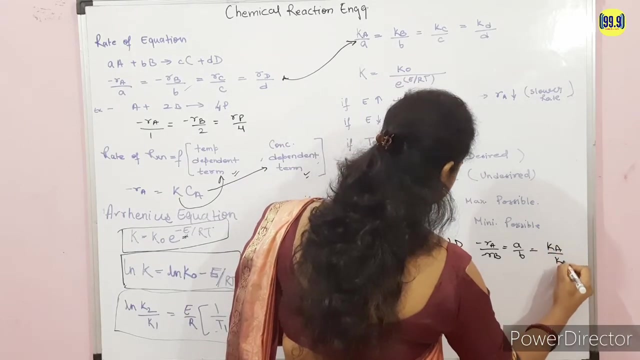 52,, 52,, 53, and 54.. If we divide equation 1 and 2, what will happen? Minus Ra upon minus Rb, and which is equal to the a upon b, and this equation become after dividing is equal to Ka upon Kb. So by: 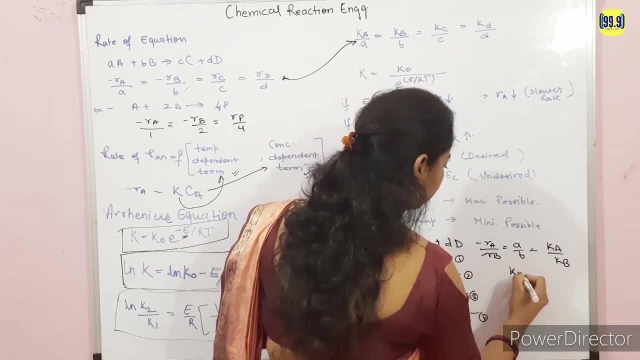 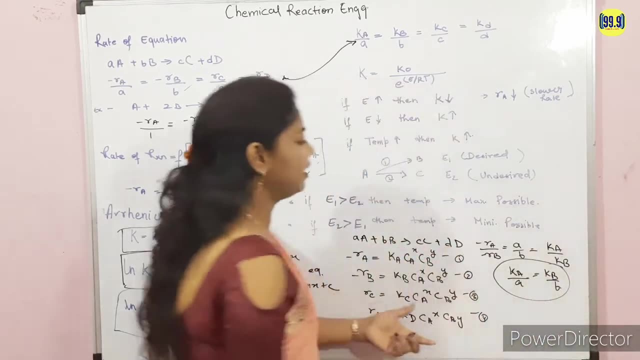 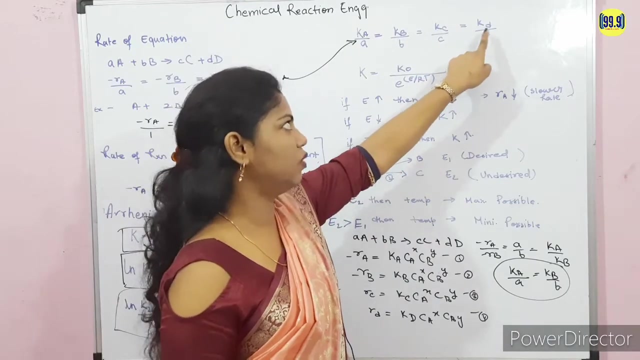 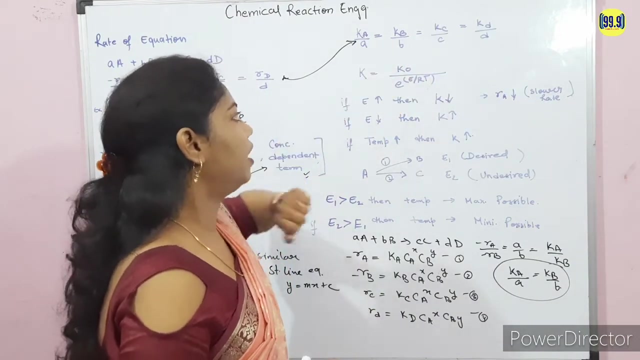 simple, simply cross, multiplying, we get the equation that is Ka upon a is equal to Kb upon b. So from here we got the relation that is K A upon A is equal to K, B upon B, is equal to K, C upon C, is equal to K D upon D. So this is also very important concept, or related to the rate of 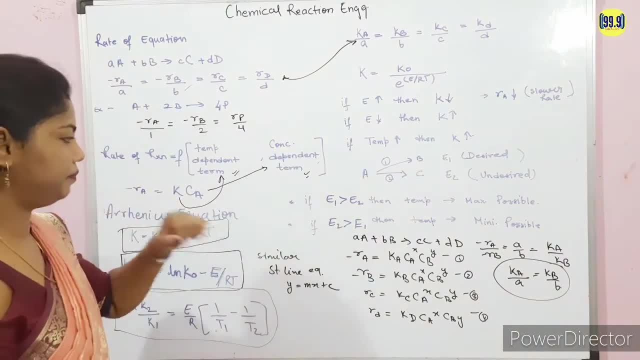 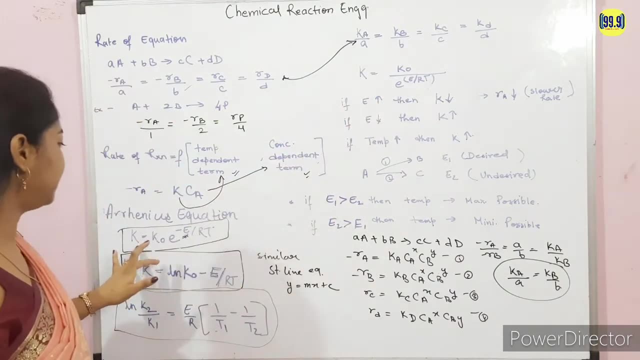 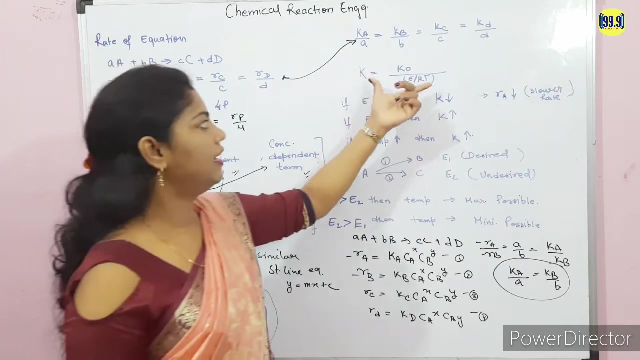 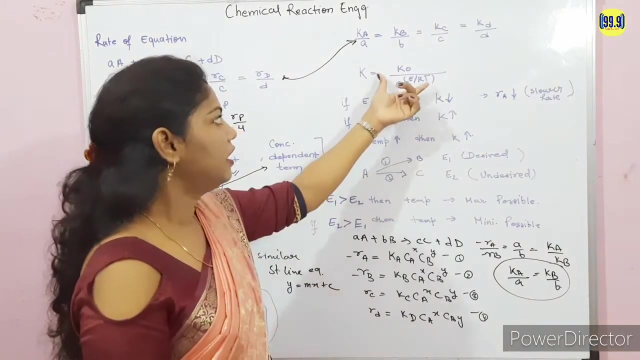 reaction. Now, as we know that the Arnie's equation, according to Arnie's equation, the equation is: K is equal to K, naught E to power minus E upon RT. So we rearrange this equation like that, that is, K is equal to K, naught upon E to power E upon RT. ok, Here the, if we study. 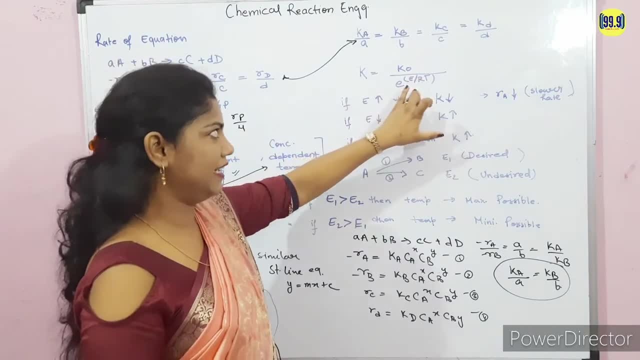 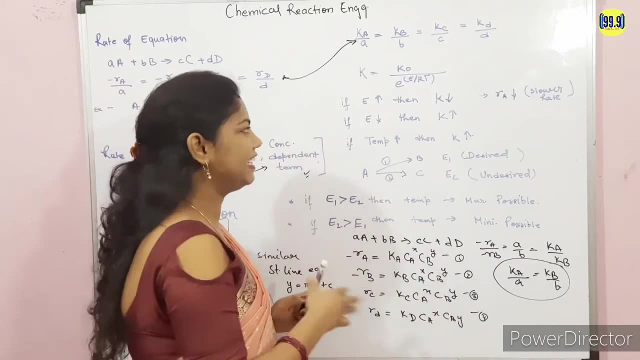 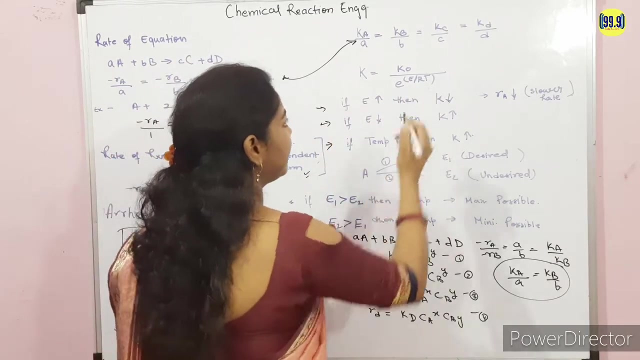 the relation with variation of activation energy. with the reaction rate constant, what will be the concept? that is, we produce a three concept, that is, number 1, number 2 and number 3.. First one is: if we increase the activation energy, what will happen? the K value is decreases. 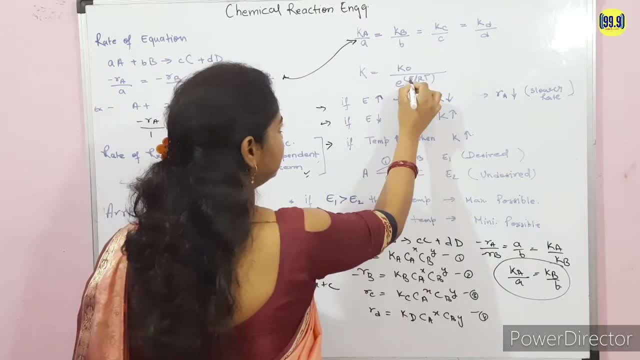 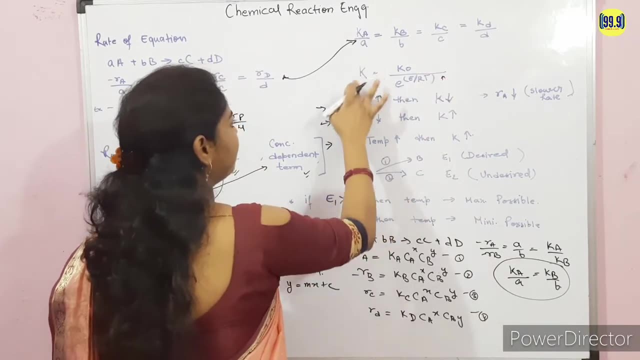 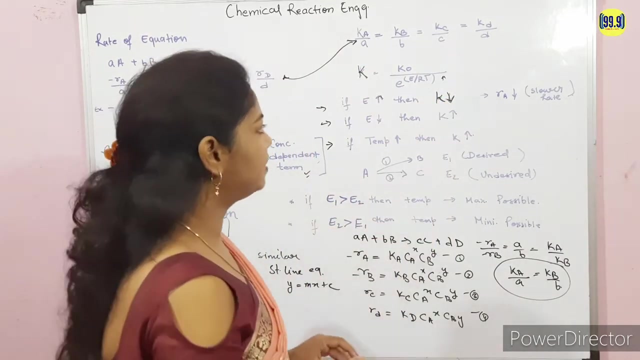 like if we increases the activation energy, the whole term is increases. ok, If this term is increasing, it means the K value is the. is K value is automatically decreases- ok, after dividing it. That is why the rate of reaction is also reaction and it become reaction. 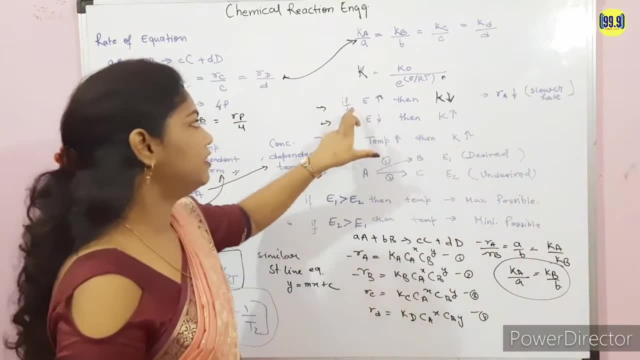 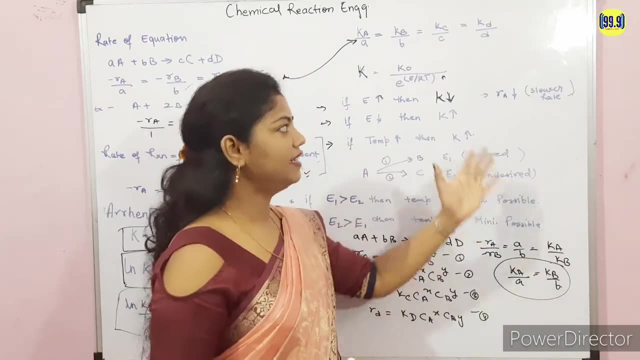 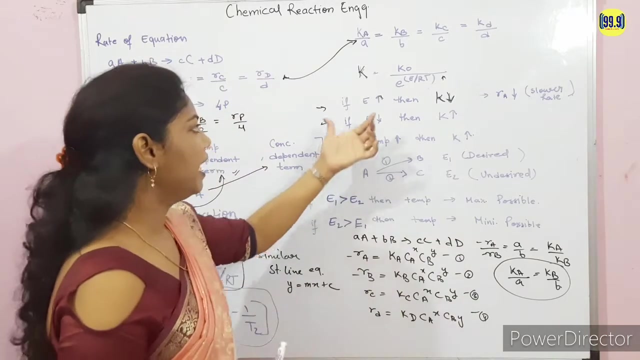 The property of the reaction rate also decreases and becomes lower rate. ok. So the concept is that when we increase the activation energy, the value of the reaction rate constant decreases and the reaction rate rate of reaction is also decreases. that is slower, it becomes slower rate, ok. Another thing is that if we decrease the activation, 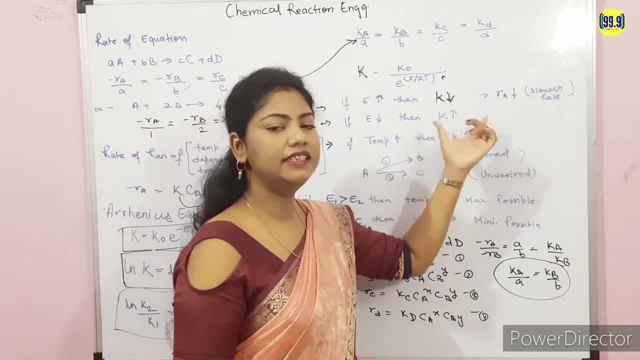 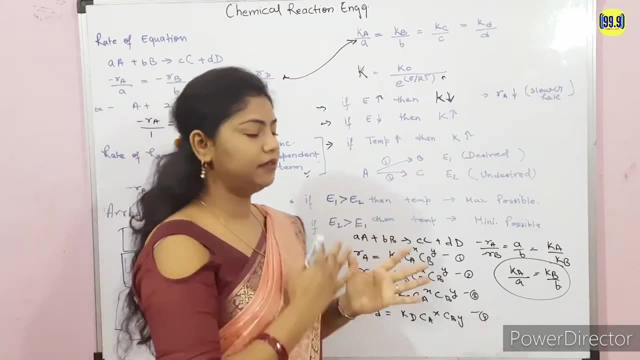 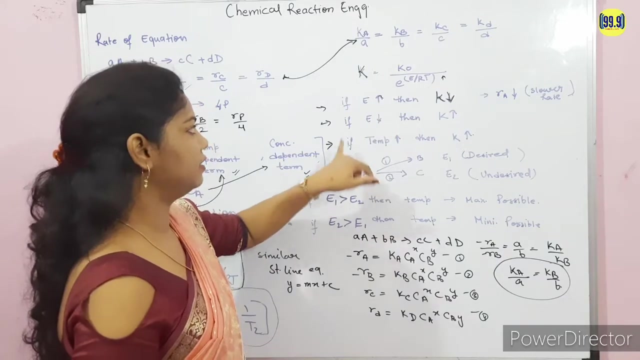 energy, the, the term that is K, is increases, ok. and in the case of temperature, if we increases the temperature then the rate- reaction rate constant- is always increases, okay. So these three term, these three point are very important for solving the gate problem and one of the trust me student. 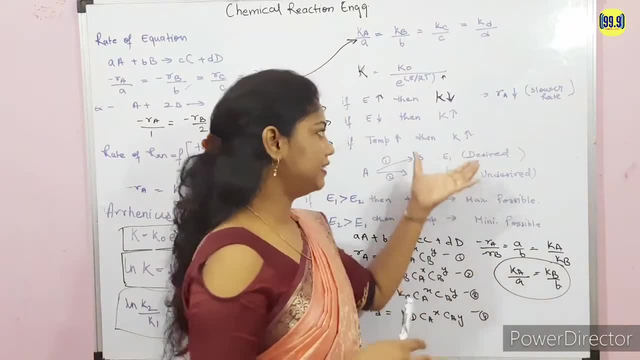 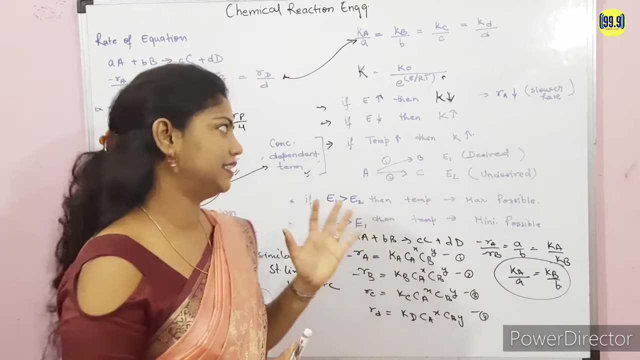 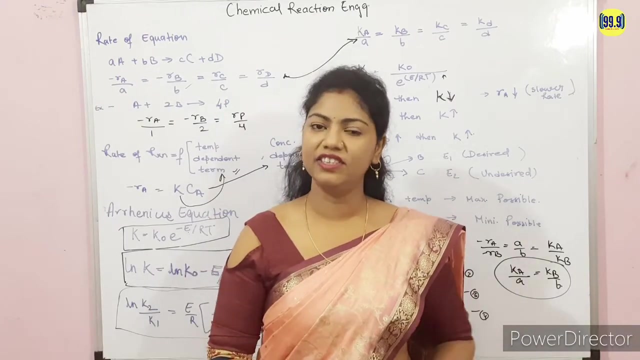 only most of the time in the gate exam. the concept related, the question related to this concept is always coming in the last classes, on in the last question paper. okay, The another thing which we are going to understand in this lecture, that is single reaction and multiple. 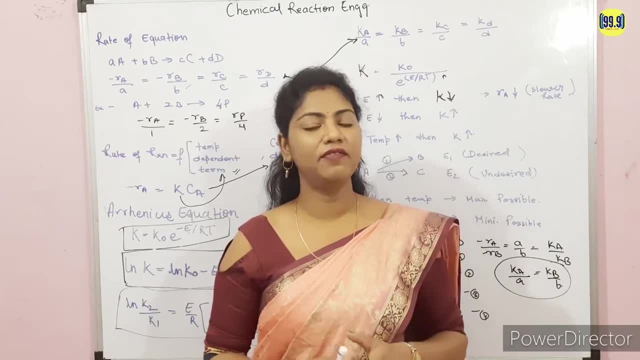 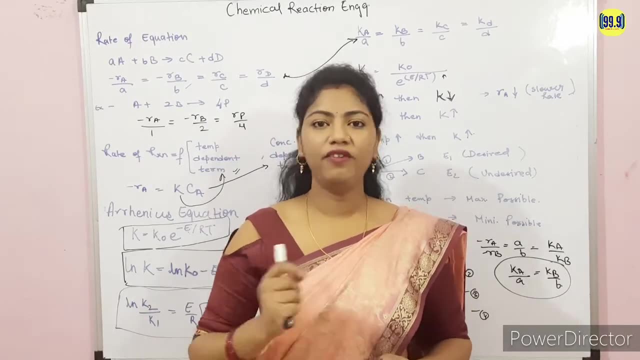 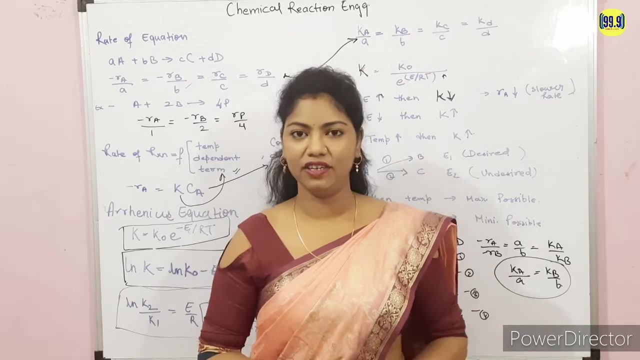 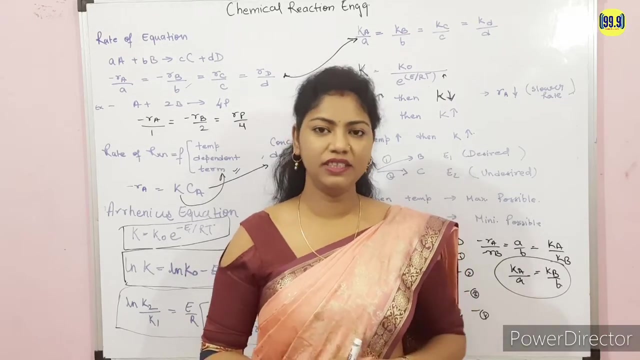 reaction. So basically, the single reaction is that type of reaction in which, when we are choosing only one statuometry equation and the one rate of reaction equation for representing the progress of the reaction, in that case the reaction is single reaction, okay. And in this multiple reaction we choose, or we needed, more than one statuometry equation. 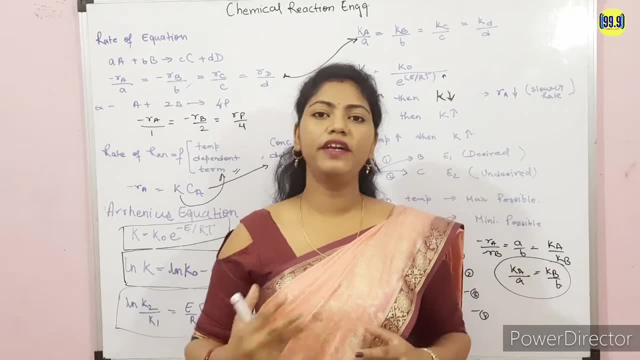 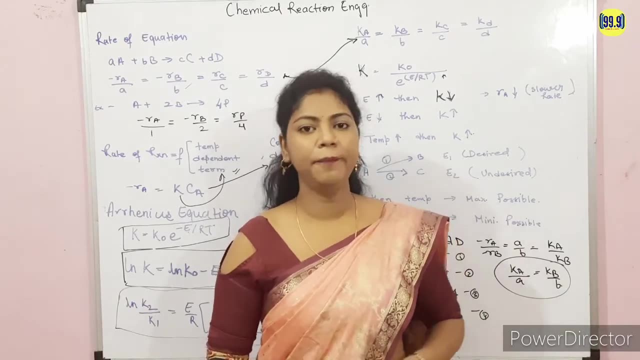 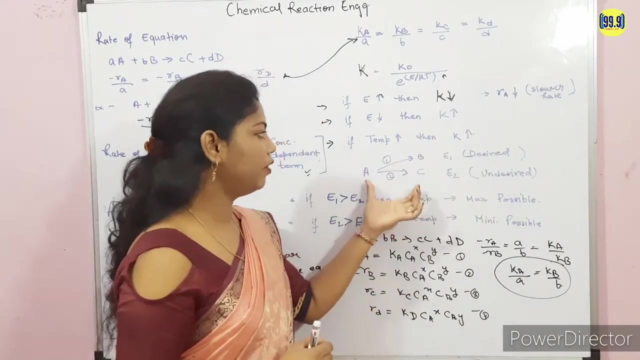 and the rate Of reaction was showing the progress of the reaction. in that case, which we call, we needed a multiple reaction. okay, So this is all about the multiple reaction, or the or the single reaction. So here I am going to show you the multiple reaction that is A gives. 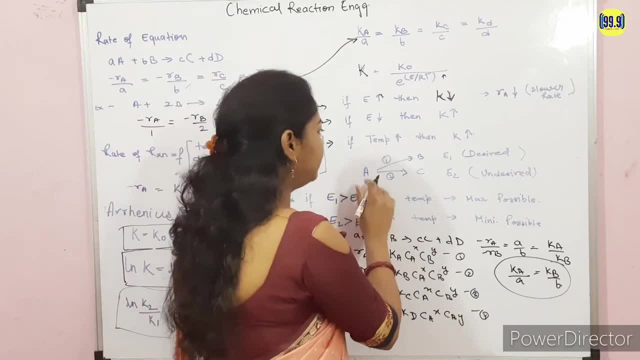 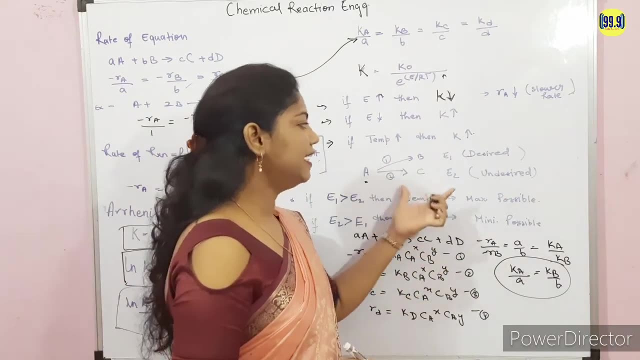 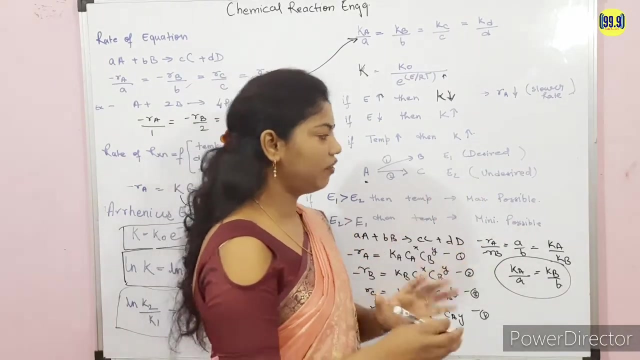 the B and C. A is the reactant, which single reactant which produces B and C. Here, B is the desired product and the C is the undesired product. okay, So activation energy of desired product is E1 and the activation energy of undesired product is E2.. So let us discuss. 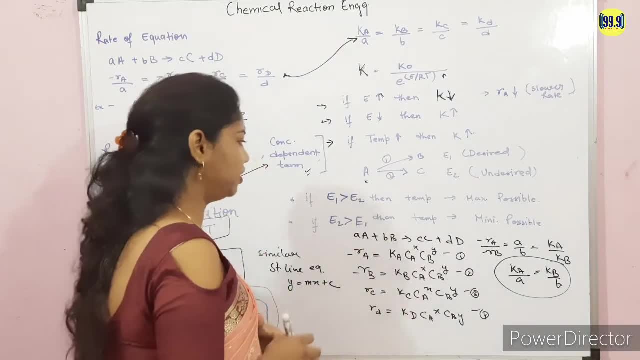 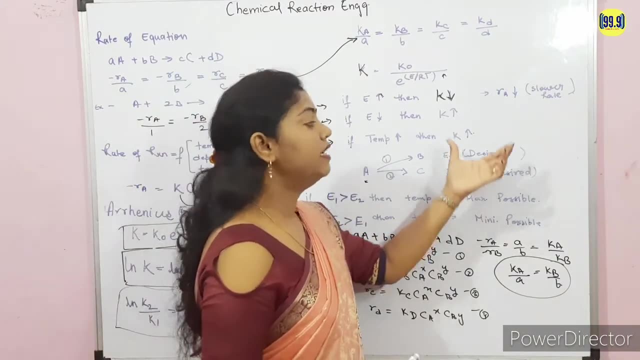 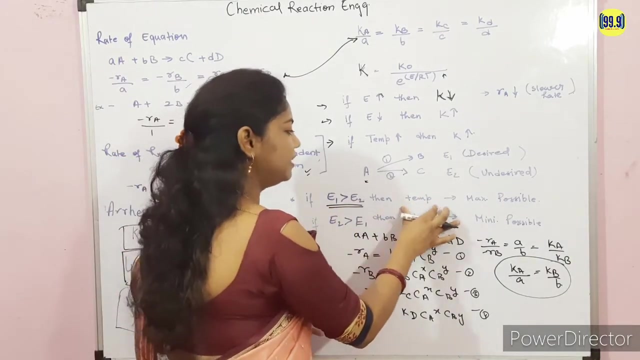 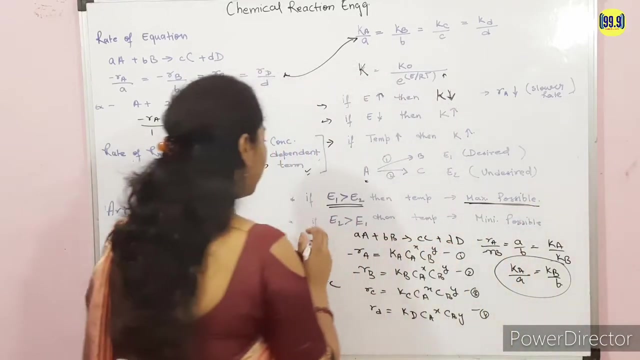 the relation between the activation energy and the temperature of the favorable temperature of the reaction. okay, So if the activation energy of the desired product is greater than the activation energy of undesired product, in that case the temperature favorable temperature of the reaction will be maximum possible. okay, maximum possible. and if the activation energy 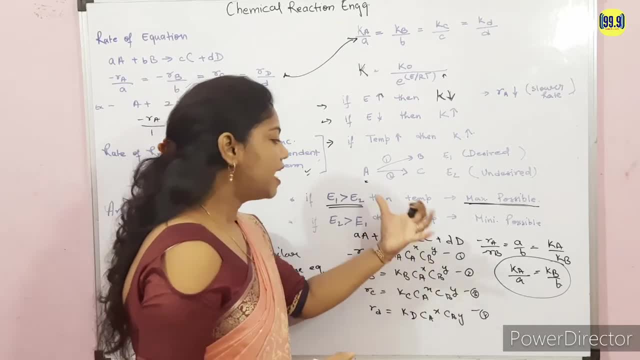 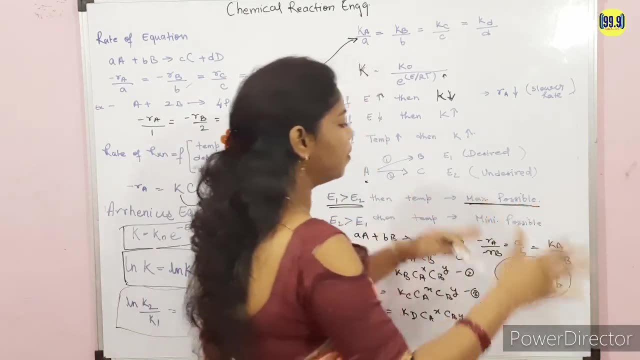 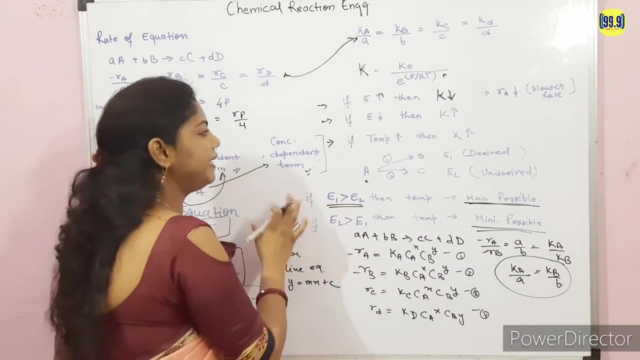 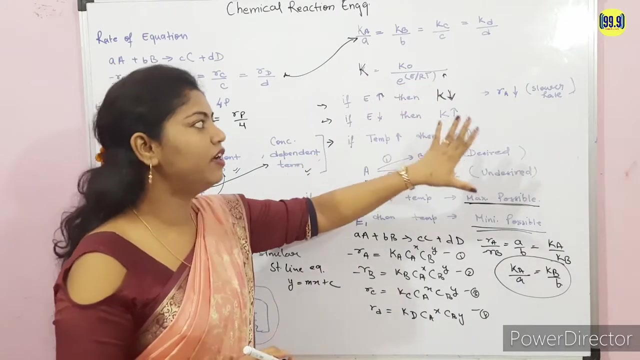 of the undesired product is greater than the desired product. in that case the favorable condition for the temperature is the minimum possible. So these two point is very, very important. it is used to Many gate problem. okay, So from today lecture we are going to, and we got the five main concept. 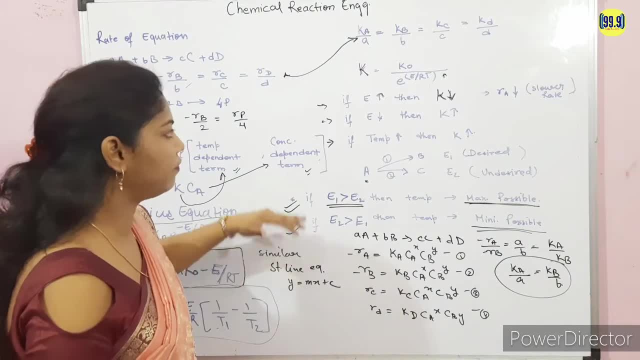 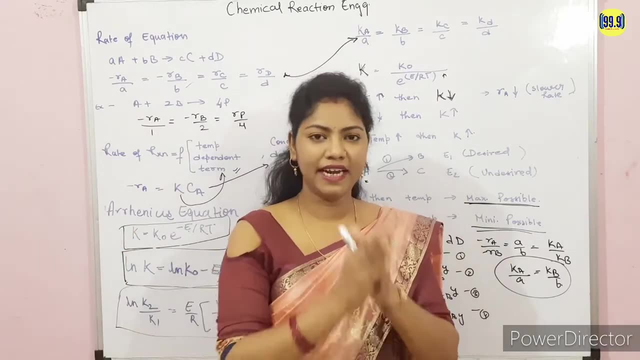 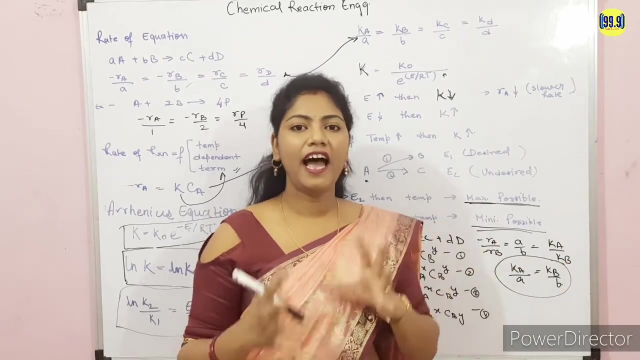 that is first one, second one, third one and fourth and fifth. So these five point are very important for solving the gate exam. okay, So if you understand today's lecture, please comment down in the comment section and please share this video with your friends, family and other students, okay. 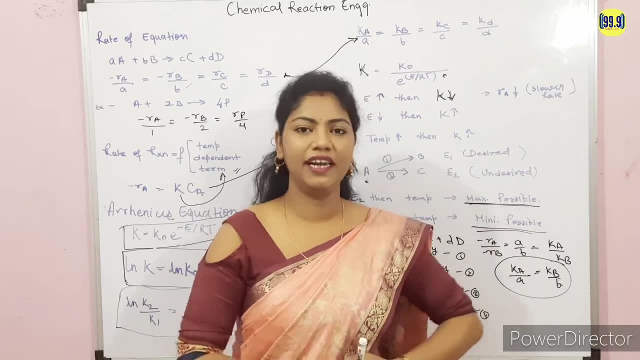 So that everyone get The advantage of this lecture. okay, So have a nice day. thank you, and have a nice day.